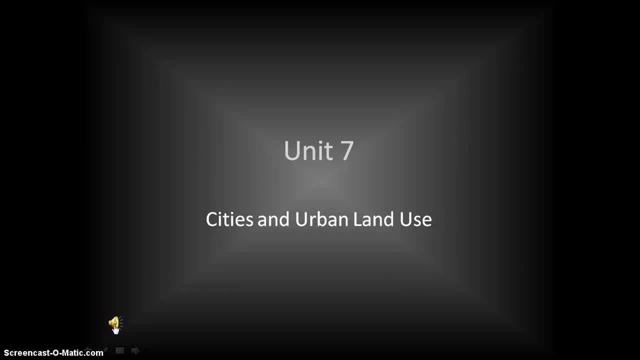 Hello everyone and welcome to another session of AP Human Geography with Mr Elrond. Today we're going to continue on to Unit 7, discussing cities and urban land use, And so in our last, previous last couple of videos, what we were looking at is kind of this trend of cities. 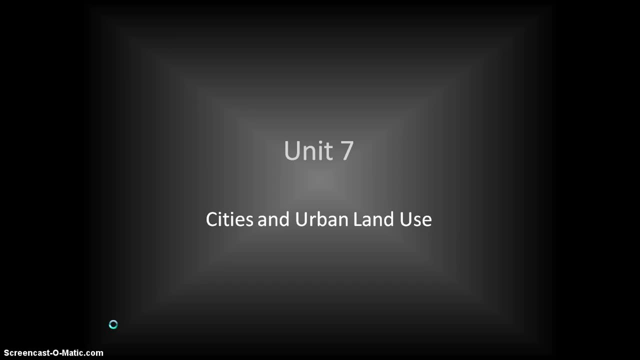 over time, geographic locations, ties to economic production, those types of things- And today, what we're going to be looking at is a concept or idea that's been developed that was called urban systems. So really, when we talk about urban systems, what we're looking at is the 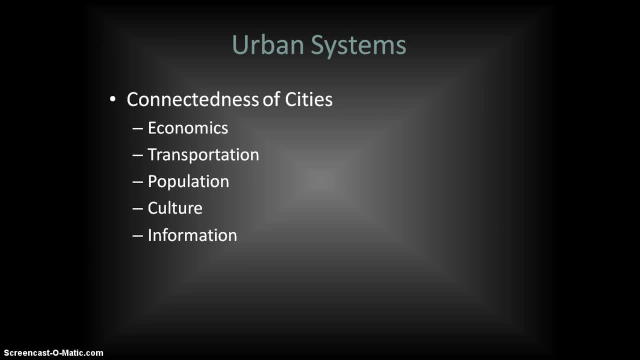 increasing connectedness of cities, And so we've been talking about this idea of globalization throughout the entire year, And so what's happened is over time. with globalization, the increasing connectedness of places is that these cities are really what are connecting each other and connect people around the world to each other, And it's really through these 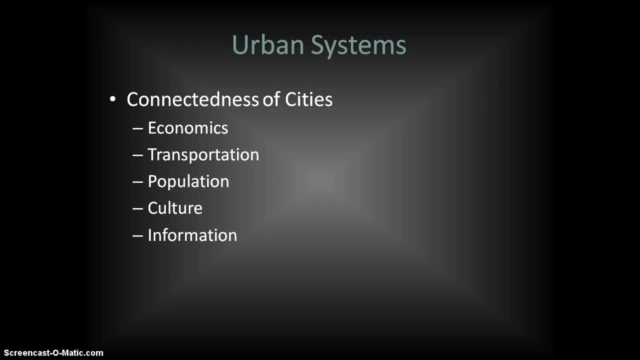 different cities, And so globalization, I guess you could say, is almost propagated through the cities themselves, because the cities almost act as the node or the center of the connection, And so not only do you have the people interacting with each other, but the cities themselves, 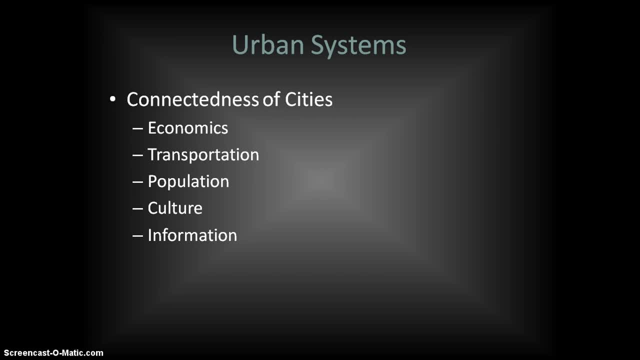 interact with each other, There's a great amount of influence on what they're doing, and so we look at the increasing connectedness of the cities, whether we're talking about the increasing economic connectedness of the citiesconnectedness through transportation and transportation methods, the way that the 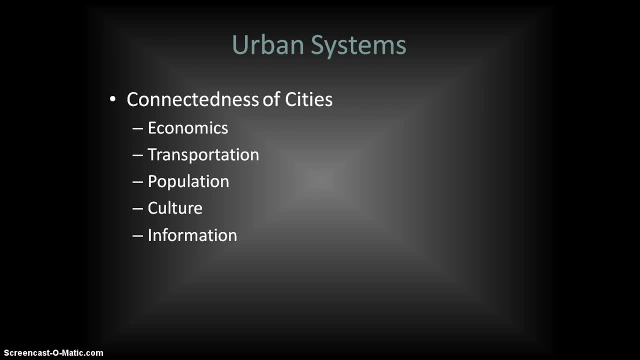 population themselves are connected, the way that they defuse and connect through culture, the way that they connect and share information, And so again, as globalization continues, you have these urban systems created through this connectedness, and the systems basically show just how are. 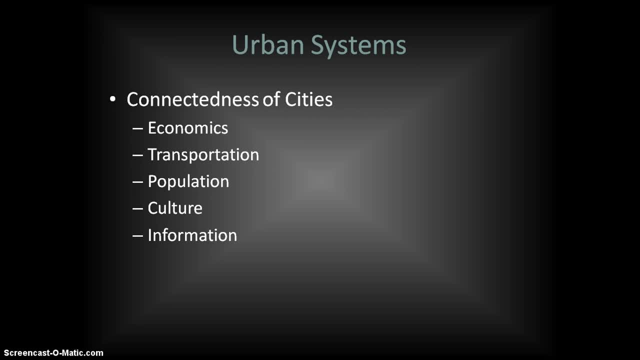 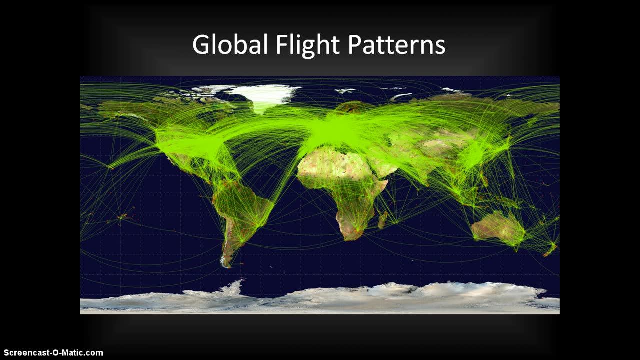 these connected and really, which cities are the most important when it comes to these various connections? so one of the things that I did is I went, found this particular map that shows these global flight patterns and, of course, you know you look at this, you can't. you can say, okay, that's great, but what you have to 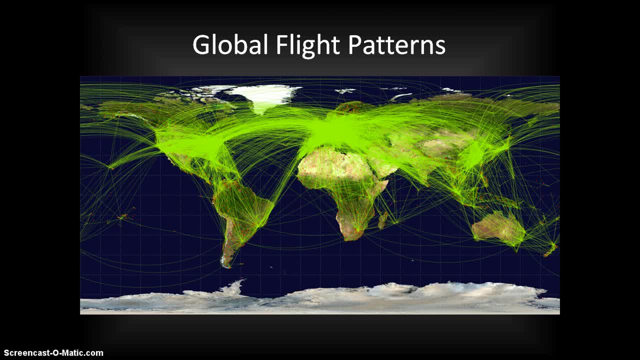 think about is the places in our world. they're gonna have airports- okay, so those are going to be more important cities that they have an airport. but then you also look at where are the flight patterns going. what places in the world are connected to each other? how connected are they? you know how many? 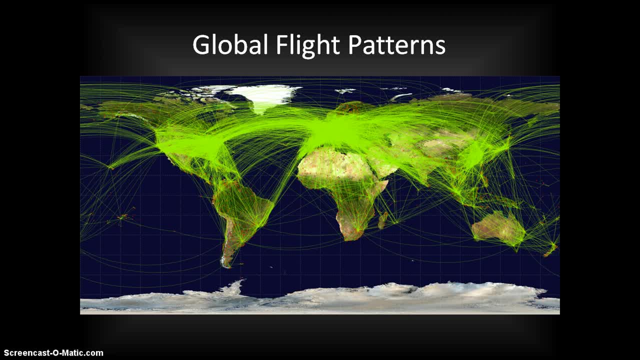 flights are making their way from one part of the world to the other, and so what kind of an influence is that going to have on that particular location and the connectedness of those two locations? and so it's interesting to look at. you know, where do flights originate from? where do they go to? how often do they go? 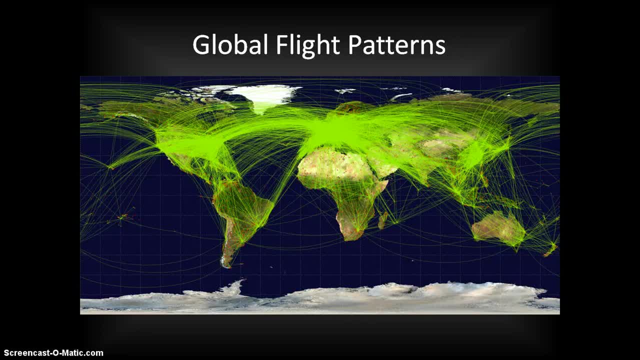 from there, and so those are the things that I'm going to talk about today: one place to the other, and you can kind of get an idea of, and get a feel for, the connectedness of those particular places, and then you can kind of do some deeper. 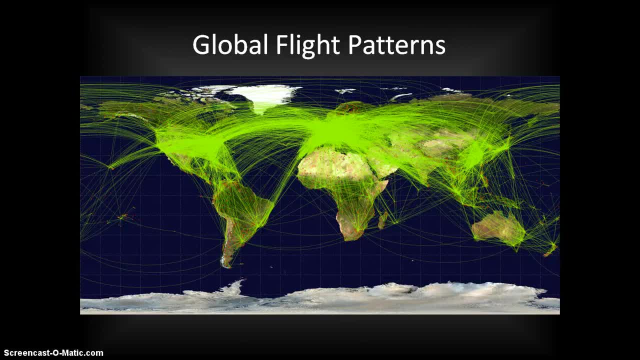 study and investigation as to you know why are not more flights going there, or what is going to be the overall impact of two places either are highly connected or you know they're not connected at all, and so I think this idea of urban hierarchy, urban systems is going to your foot- can be reflected. 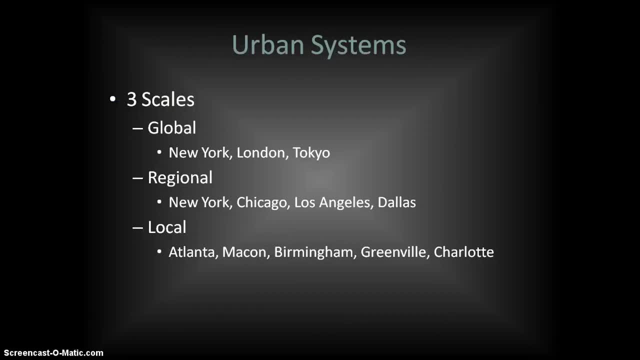 through these various global flight patterns. now, when we look at the global flight patterns, we can see that there are a number of different types of the urban system. we can basically look at the urban system as three sets of scales, and so I could talked about. the cities themselves are almost like the 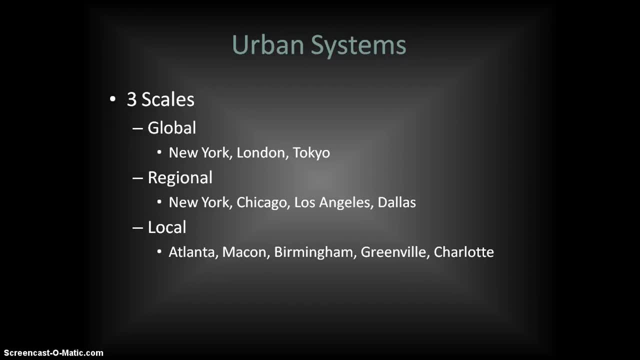 nodes of the globalization. so, as we talked about in unit one, if you remember, all the way back at the beginning of the year, we did talked about different types of diffusion and we talked about how you know, especially with cultural diffusion, you have these important cities where culture originates and that kind of 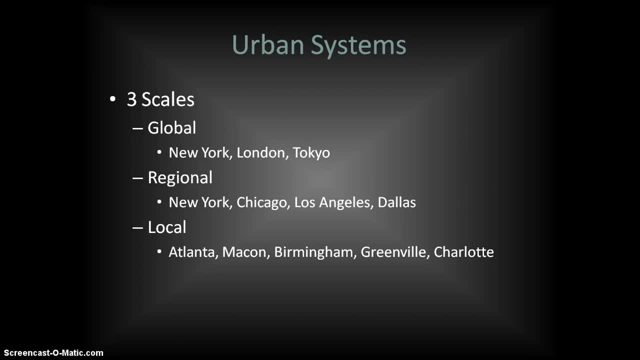 filters those way down. if you think about hierarchical diffusion, filters its way down to cities that are of less importance, and so this urban systems situation is the exact same way. you have the cities that are of utmost importance kind of on the on the highest levels, and then you can work your way down cities. 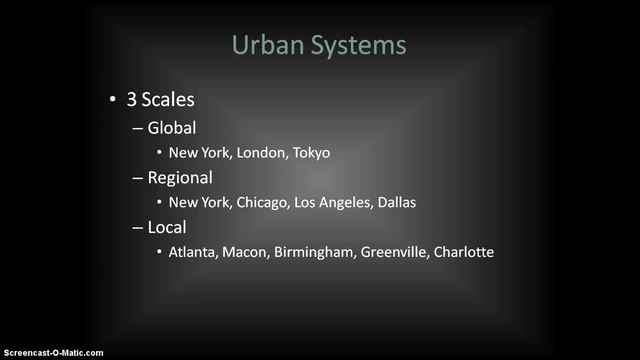 that are still important, but not as important as cities that are above it, but certainly still important for diffusing information to the, to the immediate area. so, really, like the urban systems again exist on three scales: you can look at the global, the regional and, you know, possibly the local. so of 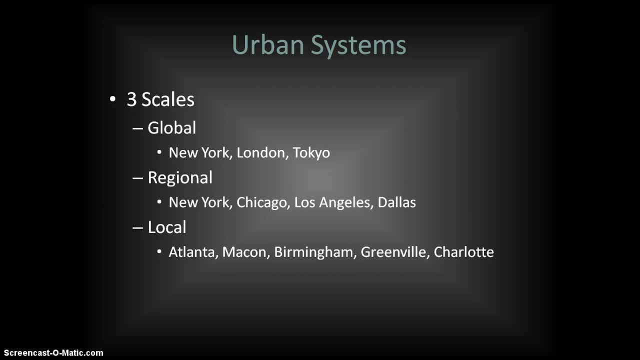 course you know you have important global cities, places like New York, London, Tokyo, places where you know the hubs for economics, hubs for culture and, in some places, the hubs for international politics. then, of course, you have regional cities that are regional importance. you look at places like New 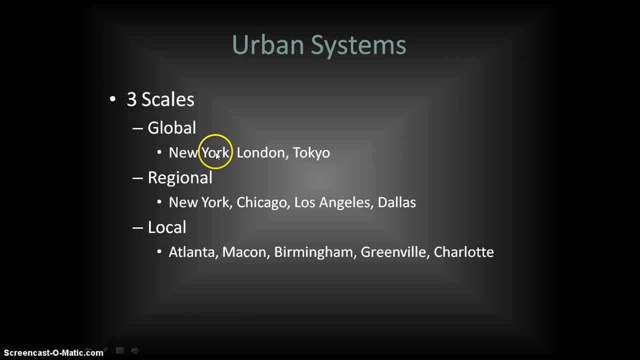 York. you know New York kind of exists not only as a global and globally important city but certainly a regionally important city among the entire Northeast. so place like New York, Chicago, Los Angeles, you know, an emerging city that's becoming more important as the city and Dallas and you. 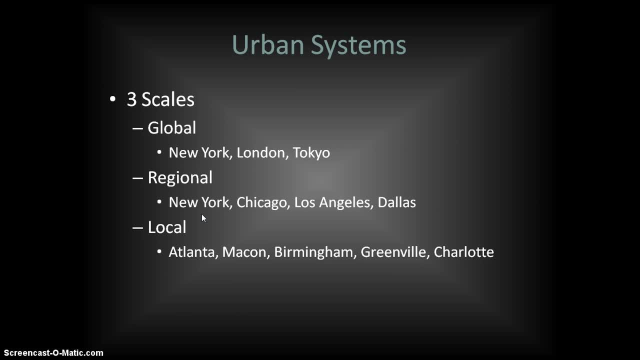 look at these across the United States as cities of importance and as information filters down from the global level. I filters down to the regional level, to these various regional cities, and then diffuses out to the cities that are not necessarily as important, and all these cities are are connected. 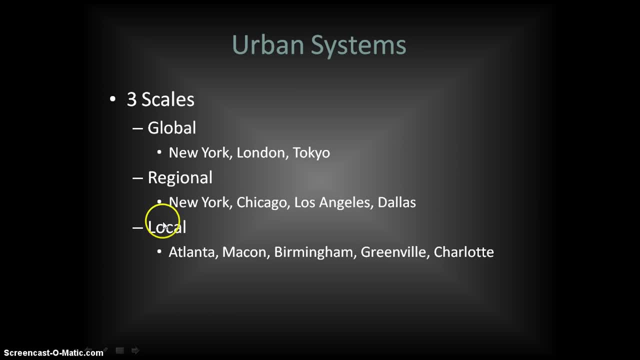 to each other, and then they're connected cities that are beneath them, and then, of course, the local level. so what happened is information filters down to the local filters, down from global to regional and then more to the local, And in this system you have the city of Atlanta. 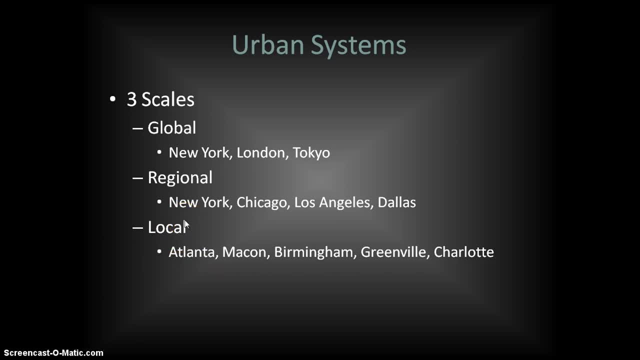 one of the more important cities in the South, kind of the hub for the South. Of course, you have the world's largest airport in Atlanta, Atlanta-Hartsville-Jackson Airport, And it actually kind of is the hub for some of these various, I guess these local cities. 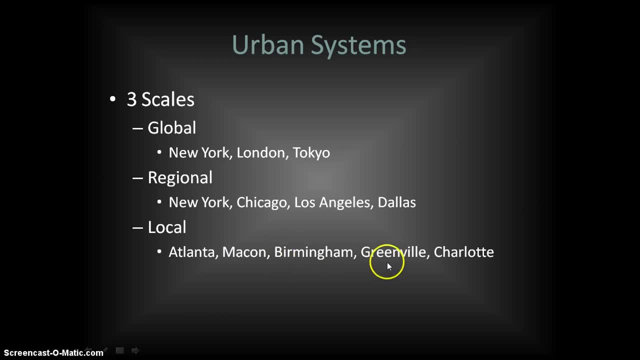 So Atlanta-Macon, which is south of Atlanta, Birmingham, Alabama, Greenville, South Carolina, Charlotte, North Carolina- You can maybe even put it in something like Chattanooga, Tennessee, And so it's going to kind of bring those together and Atlanta's going to kind of act as the hub. 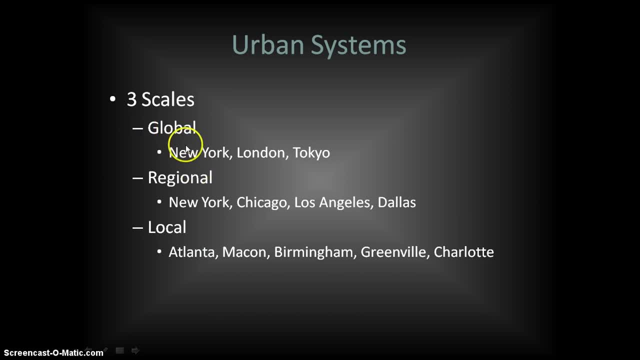 Now, certainly Atlanta does not exist on the global level, but information is going to filter down from global to regional to local, into Atlanta and then out to those other cities, And so what you'll notice is not only are these three systems connected to each other, 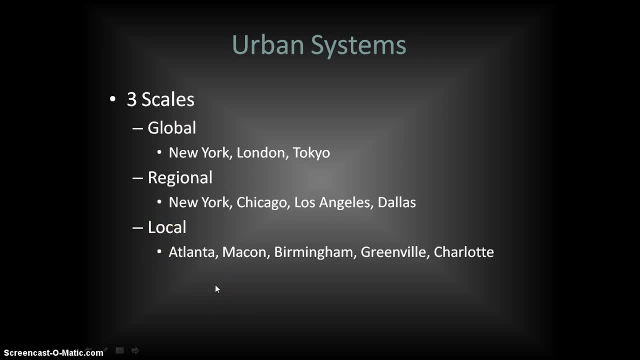 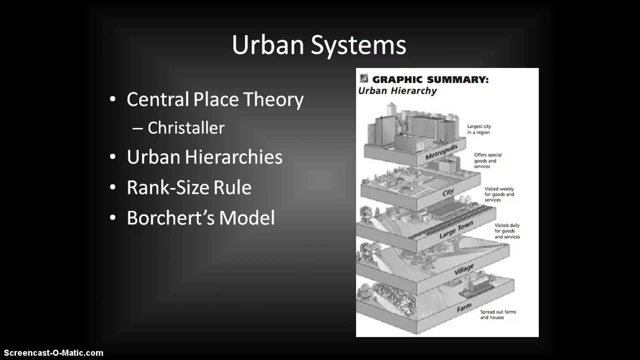 but they're also independent of each other, to where they kind of almost exist as their own network of cities. They're going to be interacting with each other Now, when we look at this, urban systems. this is just going to be the introductory video.